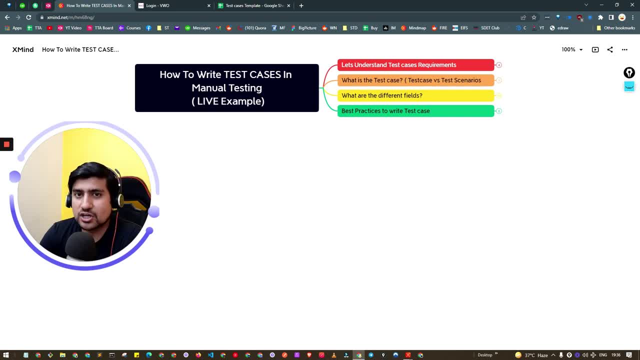 your test cases, what are the important fields in the test cases which maybe you are missing right now, or what are the best practices that I have learned personally with over 10 years experience? All right, so let's get started. All right, guys. first of all, let's understand. 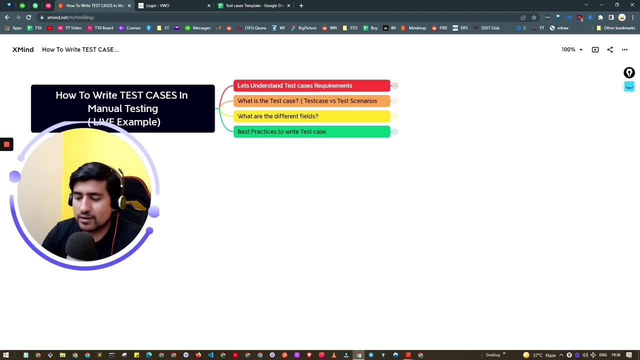 the requirements. So this is in this video, right? I'm basically taking a little different step where we will be doing live project and we'll see like example also. Okay, and I'll give you a template also that you can download and also a problem statement where you can. 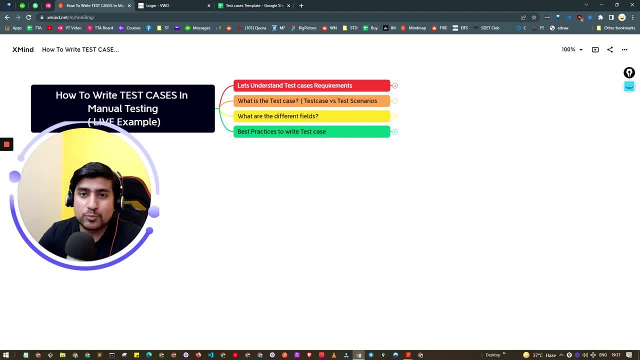 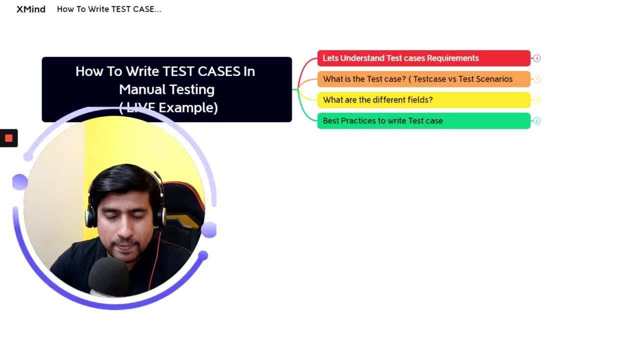 write your own test cases and I'll try to review them and you can put them into excel sheet and compile it. So comment down below with with a shared link, shared link of your excel sheet. I'll try to review them and if you're writing, if you are basically writing a very good test cases. 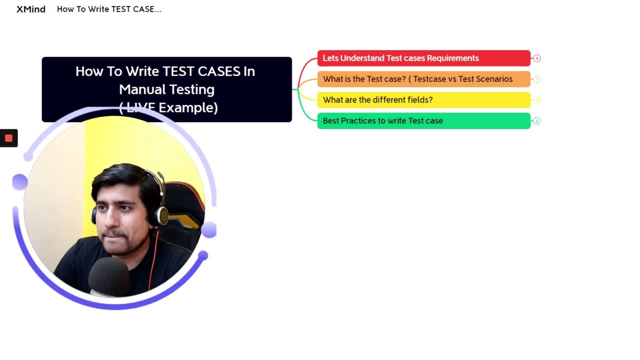 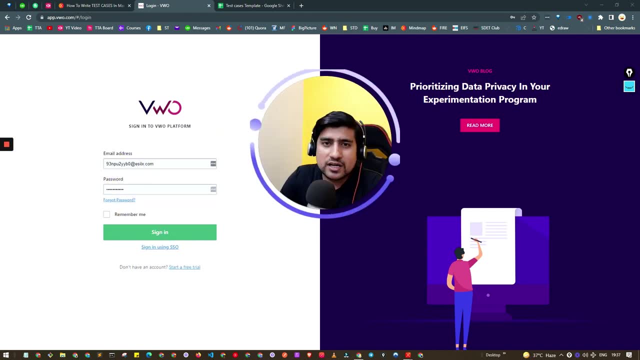 right, then probably you will get some goodies on this, Okay, so let's get started Right. So let's understand the requirement for us. So, for example, generally: so we have a very simple application, which is this one. It's a login application. It's a basically a login. 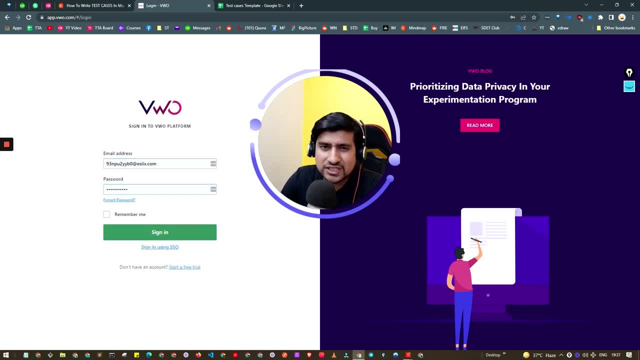 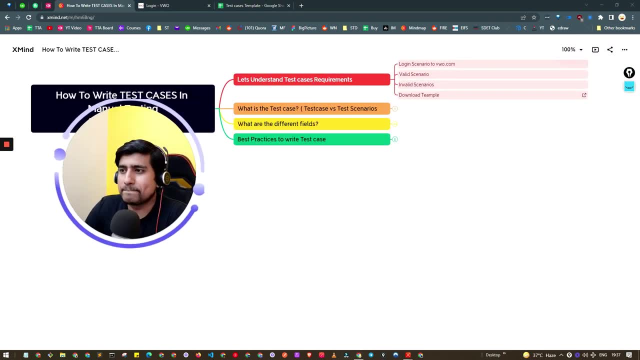 page for review to bluecom where you you can enter your username and password and click on the sign up button. Okay, So what are the different test cases that you can write Right? So this is where we are, what we are going to learn and basically, we will understand. 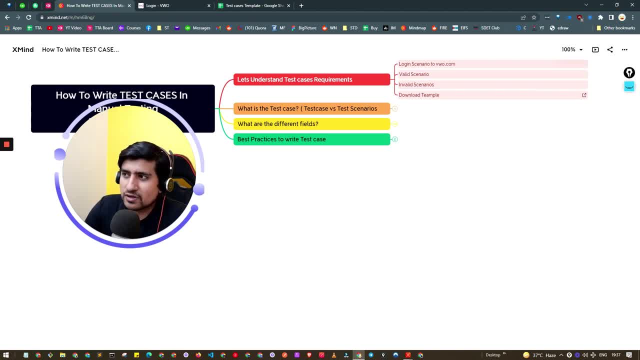 also what exactly test case is right now. Okay, so we will basically go through the valid test cases as well as the invalid test cases, and we will have a template ready for you that you can use it. Okay, the link in the description, Don't worry about it, You. 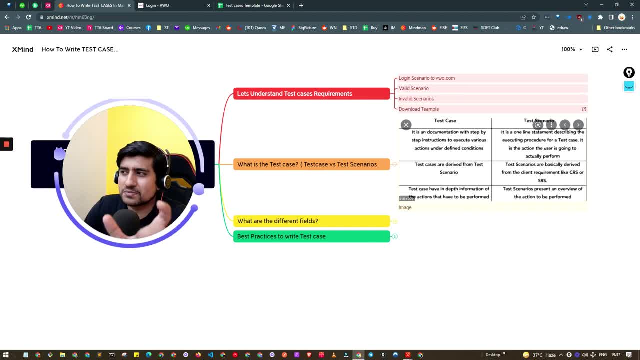 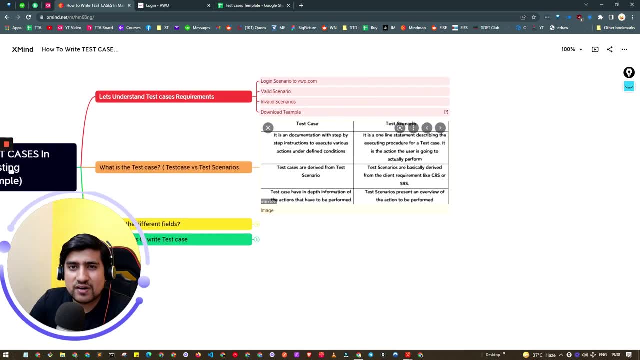 will get the link. Okay, let's understand that. test cases and the difference between test case and test scenarios, because this is where it gets confused. Lots of people are still confused exactly what we have to write in test case. Okay, so let me zoom little. 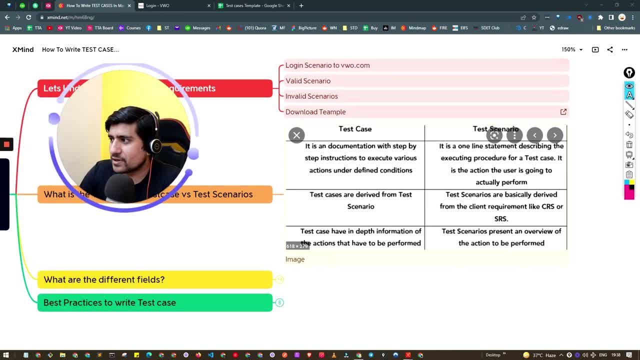 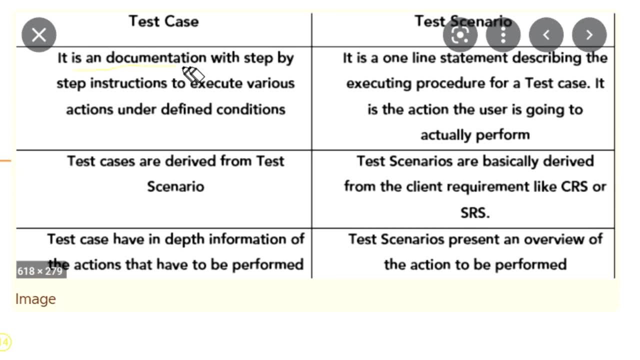 bit okay. so, if you see, let me pull up my macro post. okay, and here is a highlighter: yellow right. test case. if you see, it's a documentation with a step-by-step instruction to execute a various actions under the defined conditions. what exactly it means? let me make it little. yeah, okay, so test. 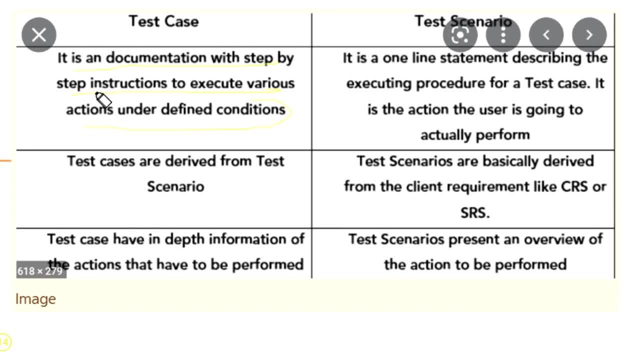 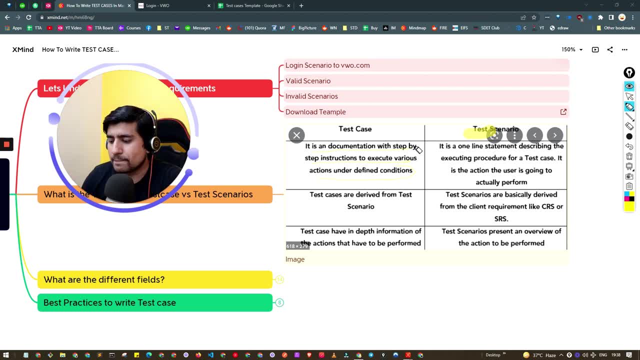 case is nothing but a step-by-step instruction to do something okay, whereas if you see test scenarios, these are just a one-liner. let me give you a very clear point with this live example. okay, now we have a login page to test. right, think about it. what are the major, or you can say, higher level? 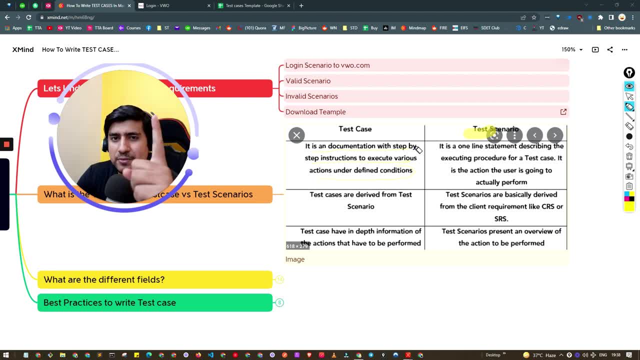 test cases that you can write. you can write with a valid test username and password and second one will be the invalid username and password. right, these are the two major important scenarios. right, you can add valid username, valid password. this is your one scenario. valid username, wrong password. 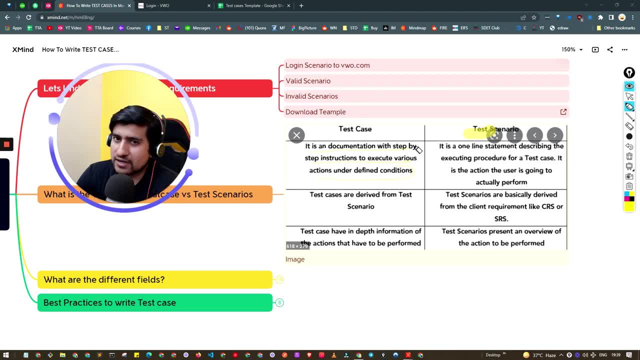 invalid scenario: invalid username. you can add valid username. wrong password. invalid scenario. invalid scenario- again invalid scenario. valid username. valid password. these are four important things that you can try out right and most of them are false under the invalid scenario and there is only one, which is valid username and valid password, which will give you a proper, positive result, which we 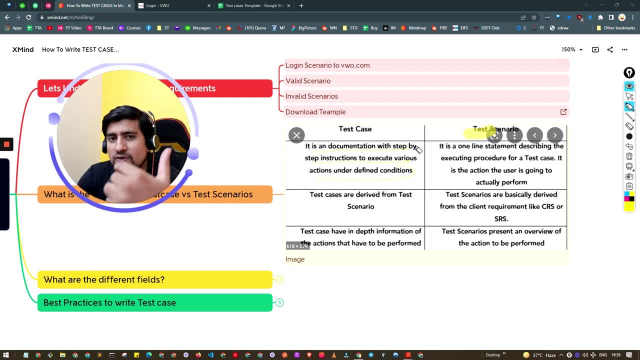 call it valid valid scenario. so we have divided high level into valid and invalid and under that we have basically two or three more cases that we have added. these are scenarios, because right now these are just one liners that we have added. now, what about the proper instruction? 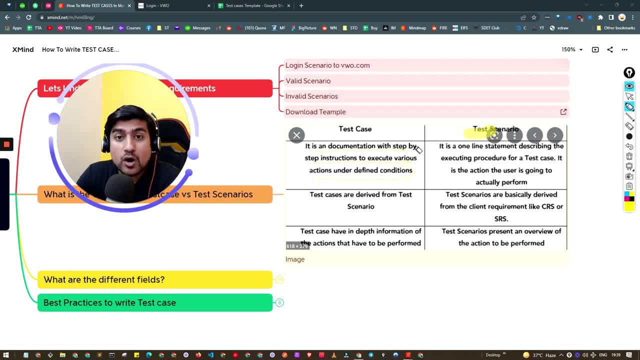 how to basically enter, what are the steps to execute, what were the actual result? what will happen if i basically do this? these are test cases, okay, so test scenarios are high level one liners and are so basically, you create test cases from a test scenarios. this is where it is important, okay. 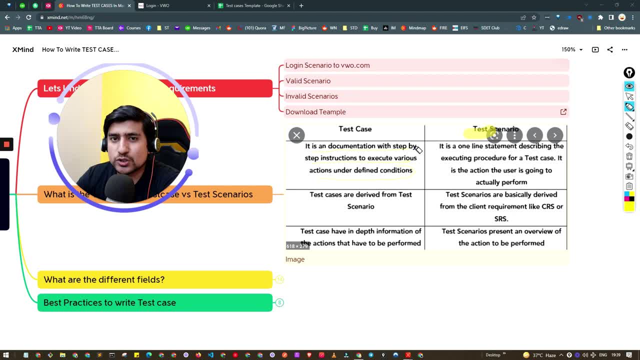 so whenever a interviewer asks you that what exactly is the test case, you can say that first of all we create a test scenarios and after test scenarios we basically take out the test cases. tests scenarios are basically created from the requirements of history, set up test case according to test seated viewer on end points. so test case with Ugh. 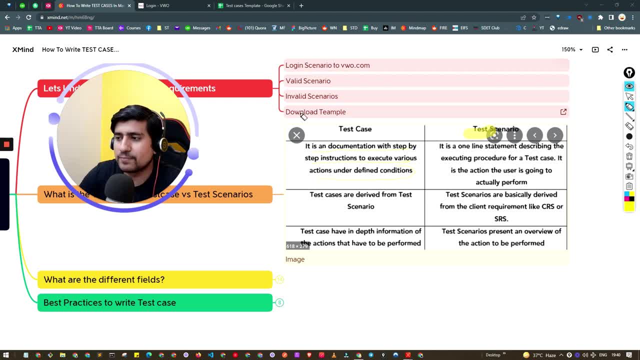 is shared. So I have shared the requirement first. right, These are the requirements. Awesome. So, if you see, test cases are derived from a test scenario. that I have told you right, And test scenarios are basically derived from a client requirement, SRS. or you can say: 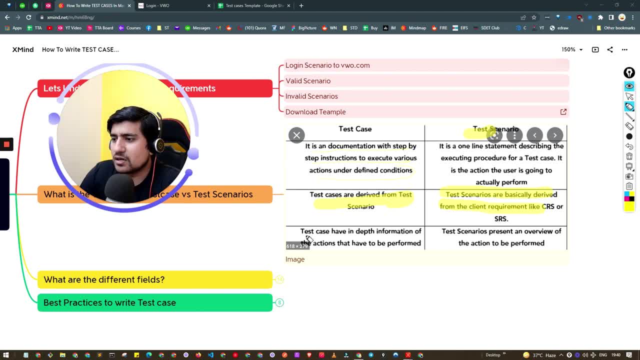 it's a software requirement or document, something like this. Test cases have in-depth information, So in-depth basically means it has steps to execute exit crit, I mean, or actual result, expected results. What are the test important fields We will discuss in this section also. 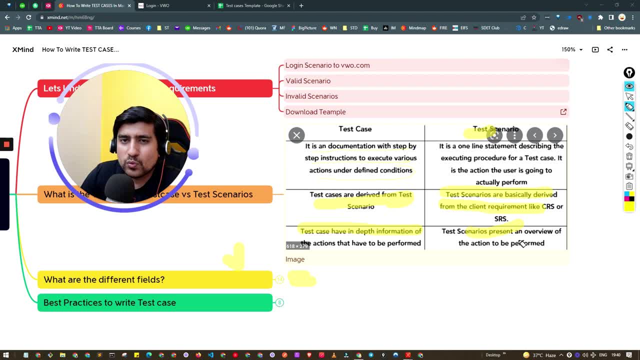 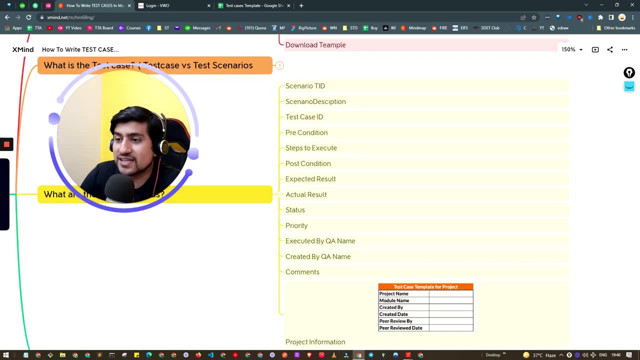 Okay. So test scenarios is just a one-liner overview What you are going to do. Clear, This is clear, Okay, Awesome, Awesome. Let's understand what are the important fields in the test cases sheet. Okay, So if you see, first of all we have a, let me, let's take it at yellow. 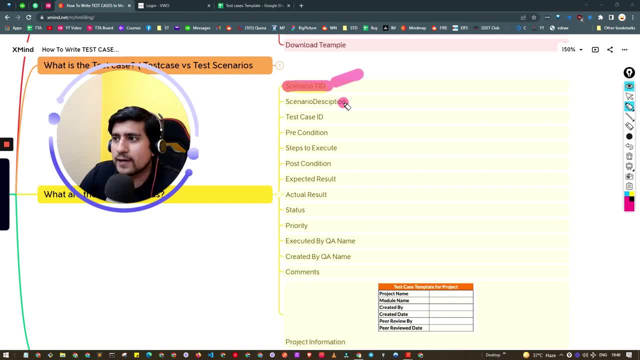 So we have a test ID, scenario ID. You can say: test scenario ID. We have a test description. You can write it out, your description also. We can have a test ID. Precondition is important, So I'll mark it. Test steps to do this is important. 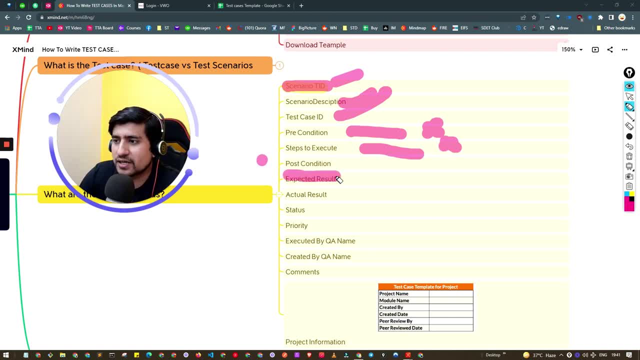 So I'll mark it as star Post. condition is important. Expected results is important. Actual result is important. Status: You can mark it Priority. What will be? what is the priority of it Is: this test case is executed by who created it and comments and you can write. 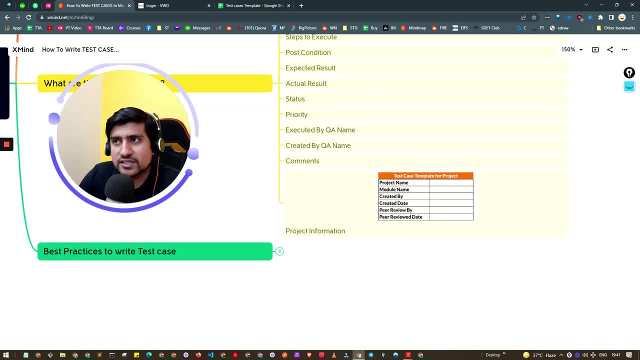 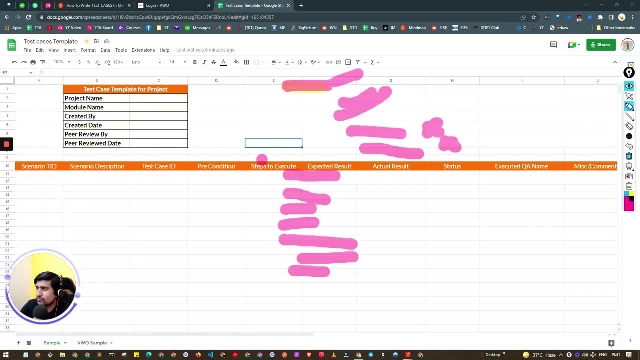 something called as a project information also Now. so let's jump into the this one sample. Okay, Let me make myself a little smaller, So here I have prepared you a template for you guys. What you can do is you can basically mention the project name. for example, VW app module name. 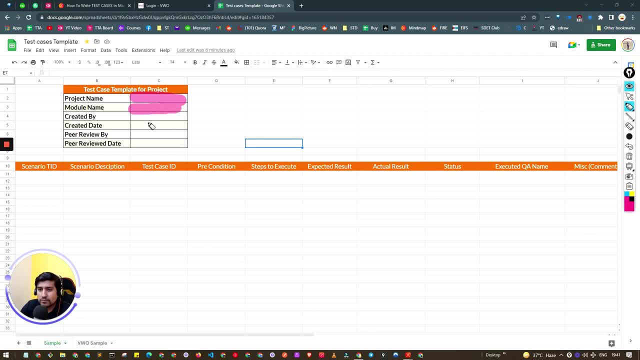 VW app is a parent Login is a module, Okay, Created by promote. created date: today's date, prior review- suppose Amit is reviewing it, or a date. So generally, test cases are getting reviewed by someone, So they we are adding it. So now we have entered all the fields that I have. 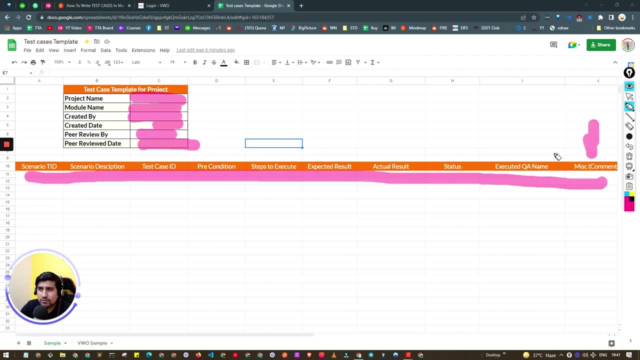 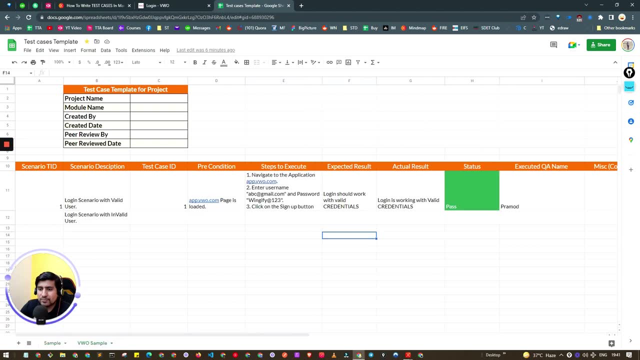 discussed with you. And last one, if you see it's a comment missed, if you want to add any information, Okay, So let's quickly create a sample for this. Okay, Awesome, I have prepared for you guys especially. All right, So this is where it comes in. 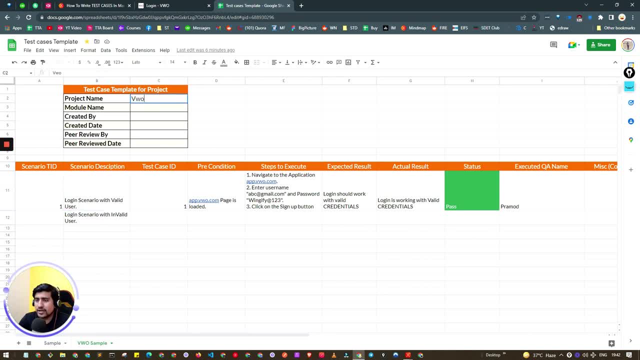 We have, I have. so basically, project name. let's do it like it would: log in, pay VW, login VW. project name is VW And let's say login page created by promote and that they can do date. I can select that. Okay, It's any, any data. I mean guys just entering any random year, 2023, don't crush me on. 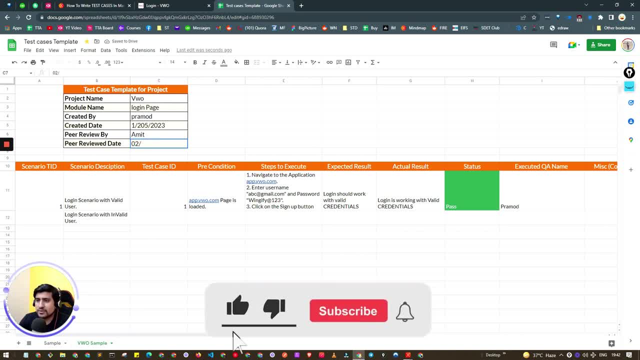 this. Okay, This is just a random date. I am ID someone from 2025 is doing it, Okay, Okay. So first one is basically login with logins. If you see, I have added a one ID login scenario with a valid. 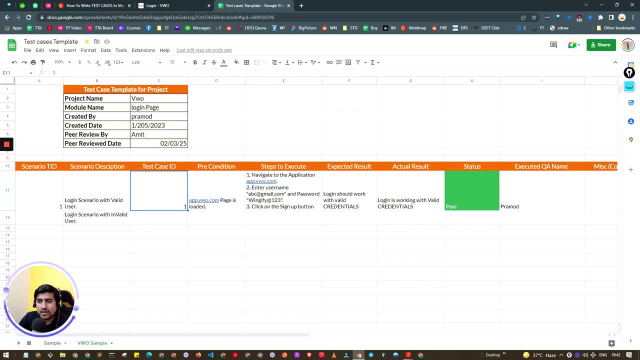 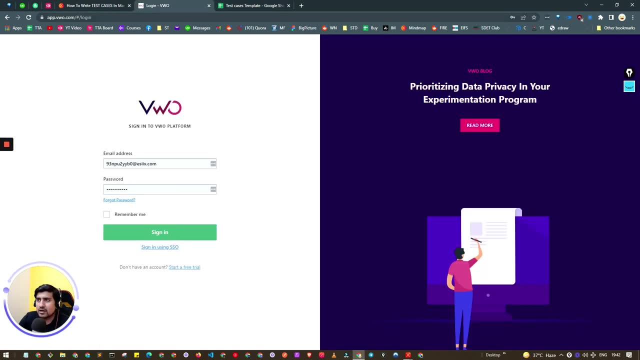 user. So I have entered a value user. What is the test case ID? I can have a one right Pre-condition: make sure that page is loaded. So page is loaded. This is like a pre-addition right And if you and so basically in this step it's to reduce, step to execute right. 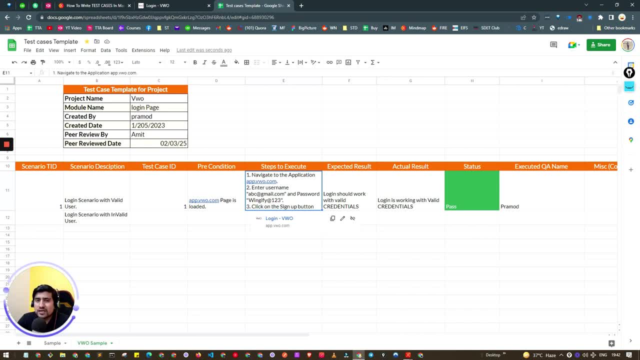 Now you have to write properly. You can write something like this, very basic, like: okay, open browser. open a Chrome browser or something like this, but this is actually expected, So you can directly jump into the, directly that browser is open. I mean, this is like a pre-condition, So that's. that's where I have. 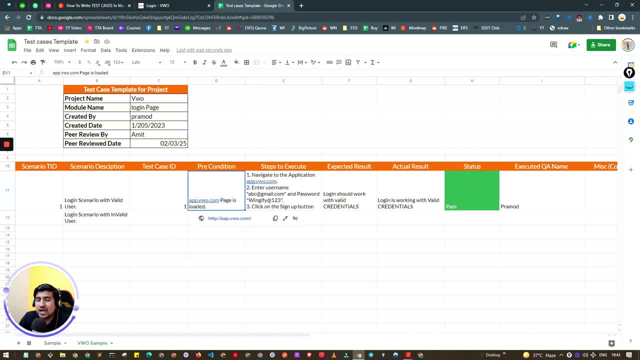 returned that it's the page is loaded. to make sure you do that, And when it is, I'm saying whenever. I'm saying pages loaded basically means you have opened a Chrome application and basically loaded a app to developercom. This is simple, right, Okay. So now basically navigate. 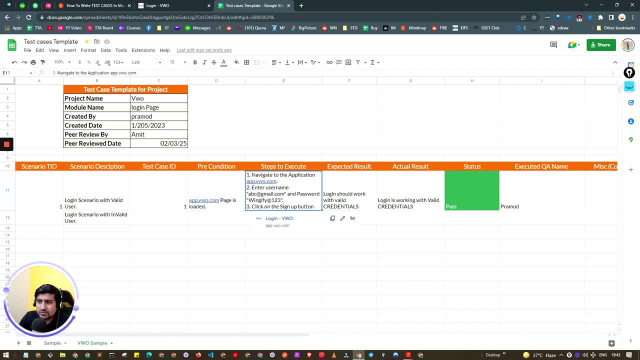 to the application, enter username, for example abccom, and password this one. So this is where it test data that I have written and it's a valid username. I am assuming it right now. It's not a valid actually. Okay, Uh, you can create a new account and it'll. 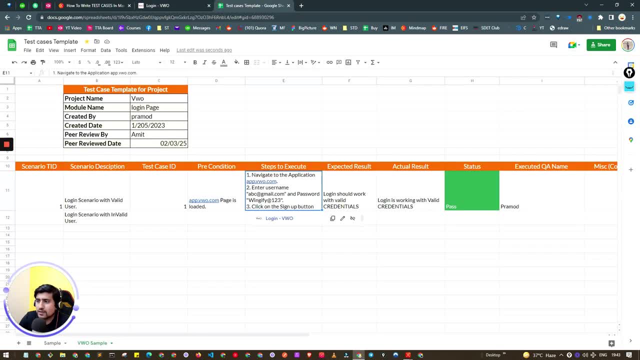 that will be valid- and click on a sign up button or a sign in button, whatever it is. Okay, Let's make it like: sign, sign in. Okay, Notice sign up button. Okay, Expected results. credentials should work. So here, if you see you I'm writing, should work. 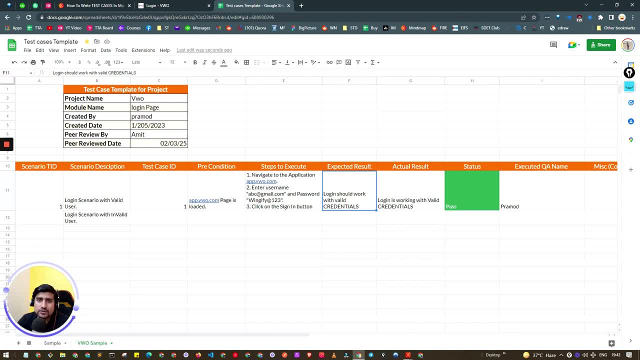 Okay, So this is whenever you write expectation: right, So it would be. it will be similar to: should. it should work, It should be this, It should be this, It should be this. And actual result is basically what happened with you. So link is working, fine, link is not working. 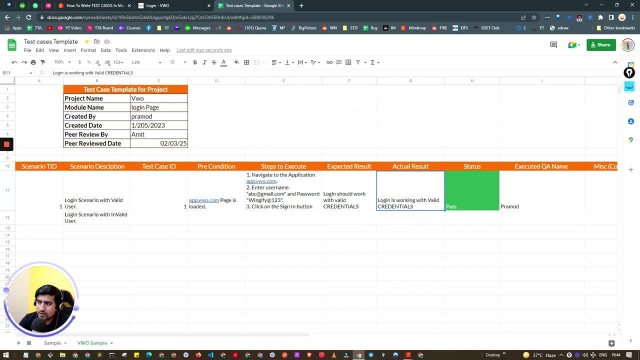 Fine link basically gives you a: so right now it's in present, Okay, And you can write it out, status or fail whenever you're running it, and you can say who executed it, or mix condition, anything that you would like to discuss, okay. so this is is. this is the live example, and now i want you to write about. 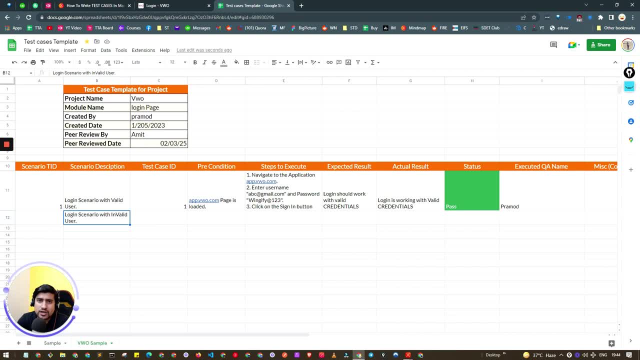 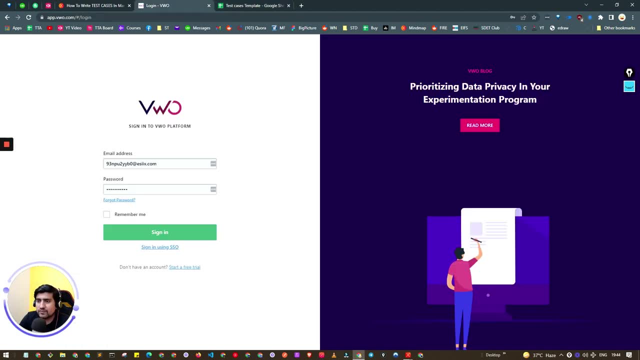 the invalid scenarios. you can write it like four or five scenarios. so you can write it out. okay, what happens if i basically enter a valid username but a wrong password, i will get a proper error. so you'll see if, uh, here i'll enter here random link, so i'll give a, i'll get a. this pop-up right. so? 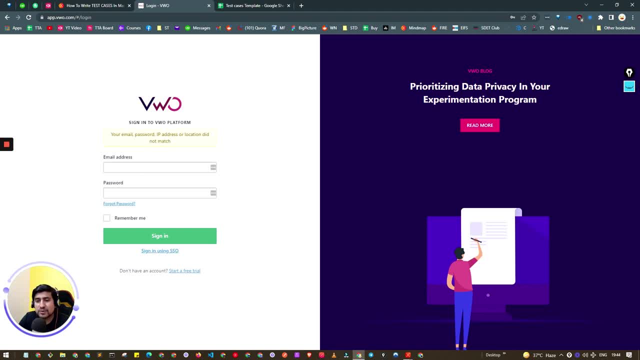 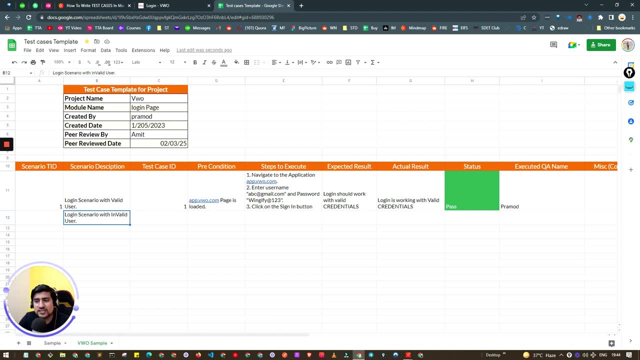 this: uh, pop-up, not, this is a message, right, so you can write it out. this is like. this is my expected condition, right? so this is this is actually you need to do. this is your homework for you guys. write it down four or five test cases. what happens if i enter a wrong username or password? right, if? 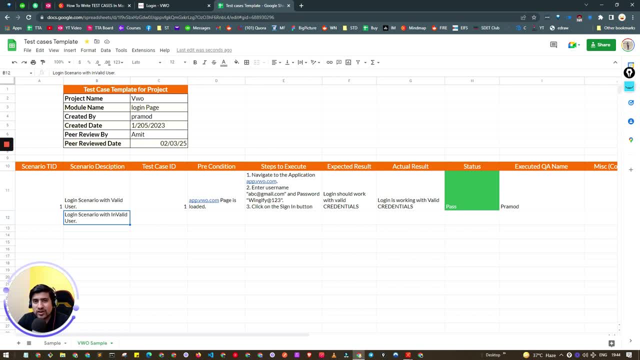 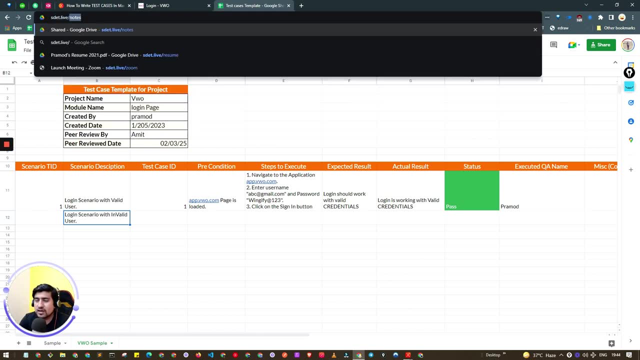 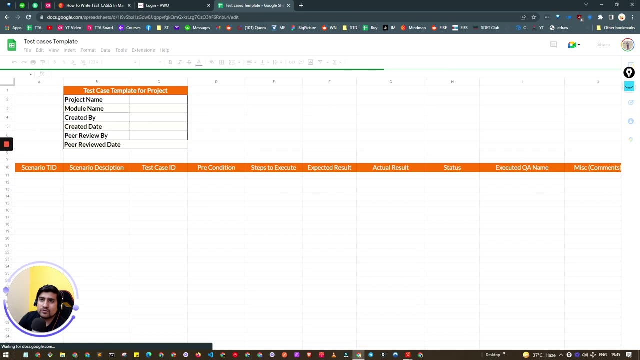 i do a. remember me what happens, right, those things, test cases. you can write it down as a practice, all right. and this template, guys, it's easy to download. you can go to sd dot, live slash, uh, tc template. okay, this link, right and you will. you can directly copy it. so just go to file file and create a copy of it, okay. 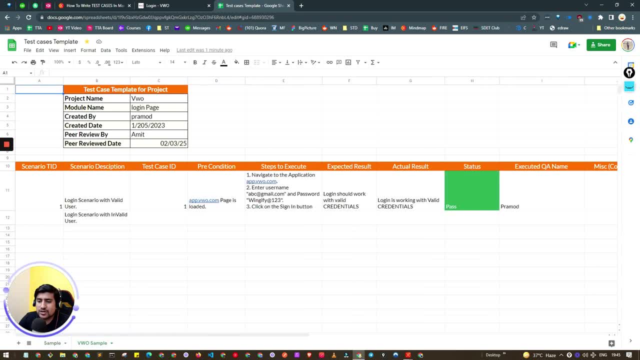 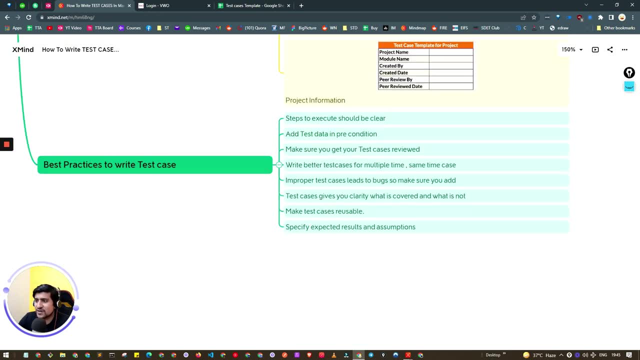 make a copy for yourself, and you can do that. there is a sample also given so you can use. reuse it, okay. all right, i hope this is clear, right, and let's move on to the very interesting part, which is best practices. all right, pay attention, guys here. make sure you are using the uh, so make sure your. 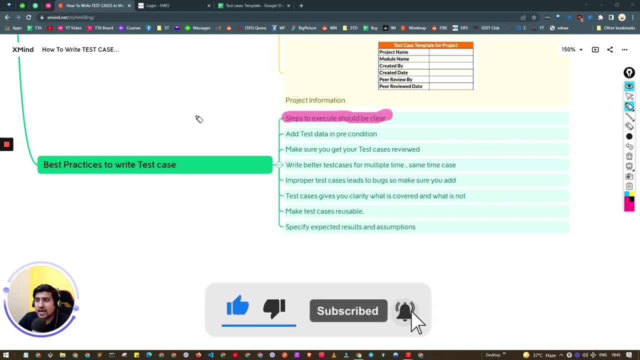 test steps to execute is clear and you basically get your test cases reviewed by someone. okay, this is very important. add test test data in the pre condition, so make sure you add test data also, what are the username and password? you can mention them because someone is going to execute it, right, suppose you? 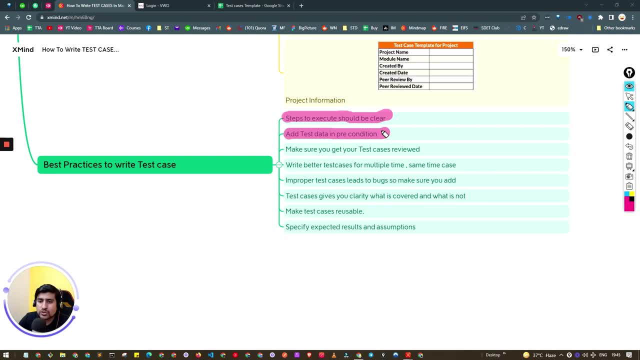 are not executing it. someone should know, like, what is the test data that you have used so you can mention that. make sure your you get your test case reviewed by someone. for example, i will, just after completing this, i will get it reviewed by amit. okay, write your test cases multi. i mean write. 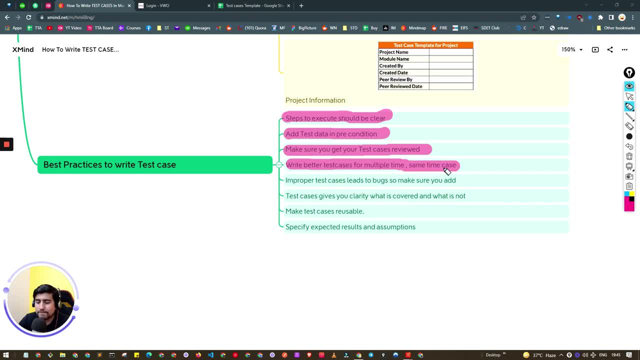 a better test cases for a multiple time at the same time case. basically, suppose you have to do 10 times a login page for a test- okay, different, you test data right, so make sure you use a proper template where you basically enter that: okay, uh, by using this 10 credentials, check the expected result, that it is working fine. 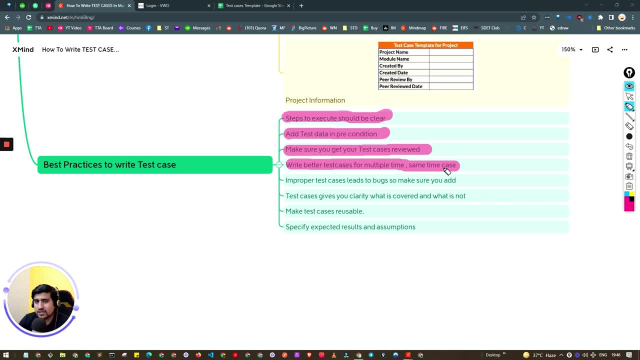 or not. okay, so you can do smart work here. the data-driven testing right. we call it data driven or excel base. so whenever you have multiple things to do with the same test case, you can say that make it like a generic use different type of test data and you can write a simple one test case and 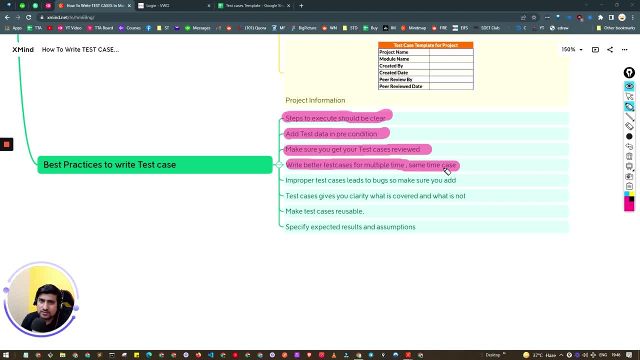 tell them that okay first and it has like five or 10 instances Okay. So that is where it is helpful. Improper test case can lead to bug. This is really important. Make sure to do that. Test cases will give you clarity and it will basically give you a test coverage- how much you have.